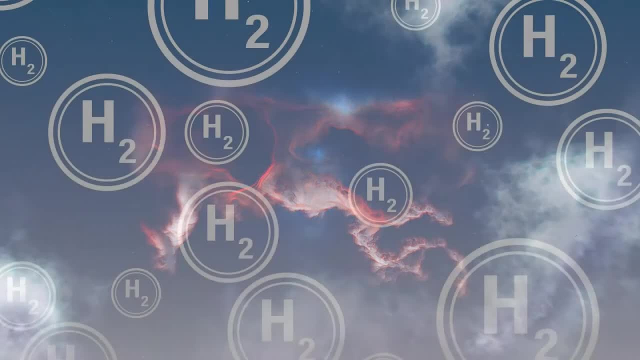 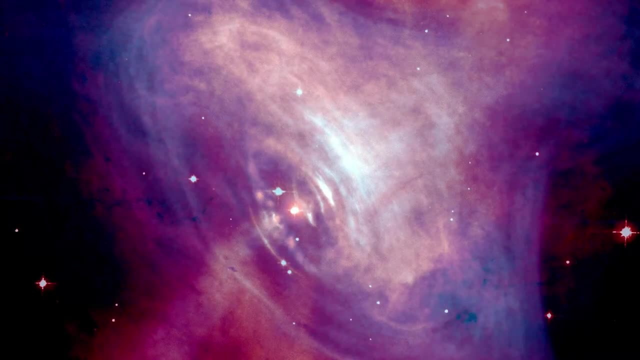 Hence it is relatively easier to measure both the amplitude and phase of radio waves – whereas this is not as easily done at shorter wavelengths. Although some radio waves are emitted directly by astronomical objects, most of the radio emission that is observed is the result of synchrotron in the blink of an eye. 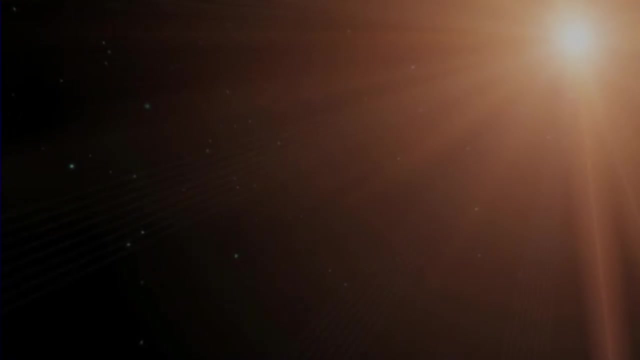 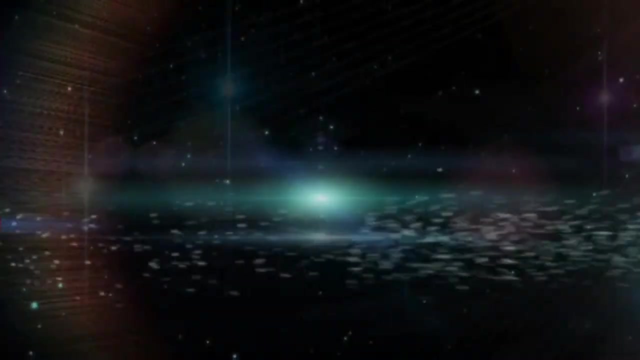 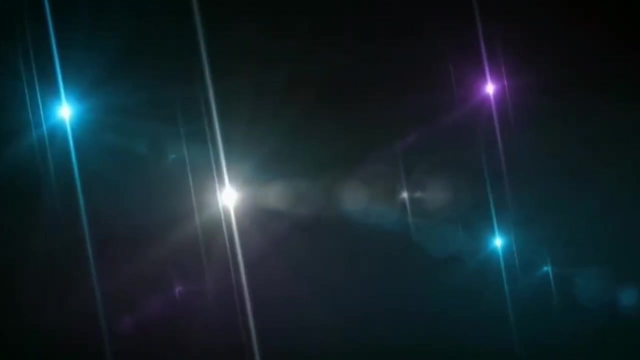 Most of the radio emission that is observed is the result of synchrotron radiation, which is produced when electrons orbit magnetic fields. Additionally, a number of spectral lines produced by interstellar gas, notably the hydrogen spectral line at 21 cm, are observable at radio wavelengths. 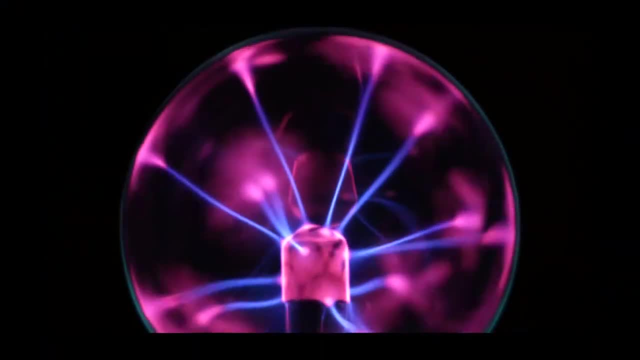 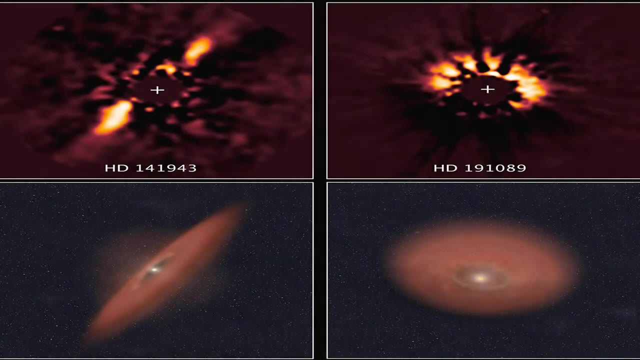 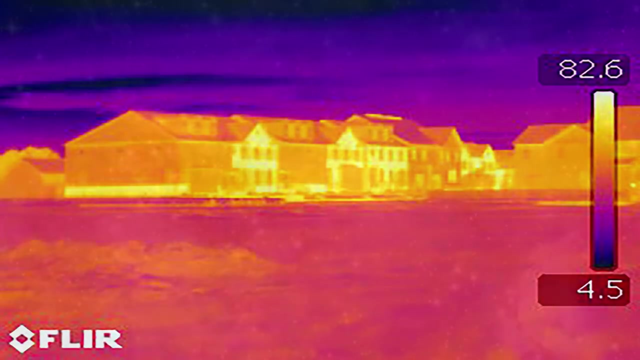 A wide variety of other objects are observable at radio wavelengths, including supernovae, interstellar gas pulsars and active galactic. nu Infrared Astronomy- Infrared astronomy is founded on the detection and analysis of infrared radiation wavelengths longer than red light and outside the range of our vision. 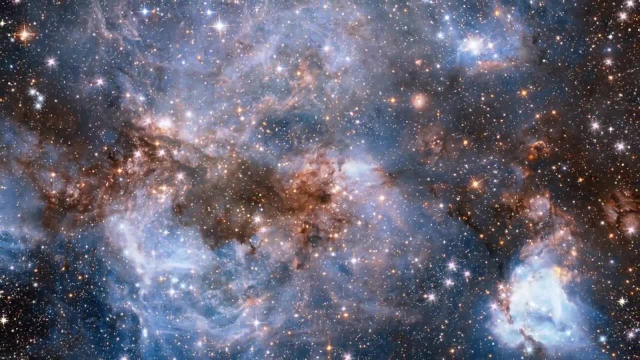 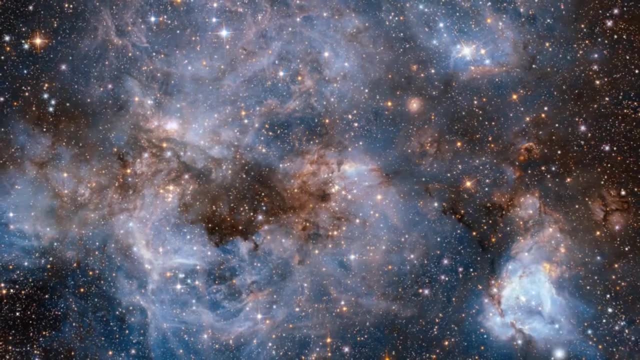 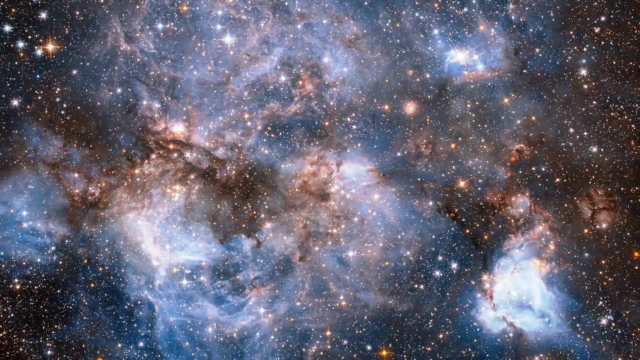 The infrared spectrum is useful for studying objects that are too cold to radiate visible light, such as planets, circumstellar disks or nebulae, whose light is blocked by dust. The longer wavelengths of infrared can penetrate clouds of dust that block visible light, allowing the observation of young stars and black holes. 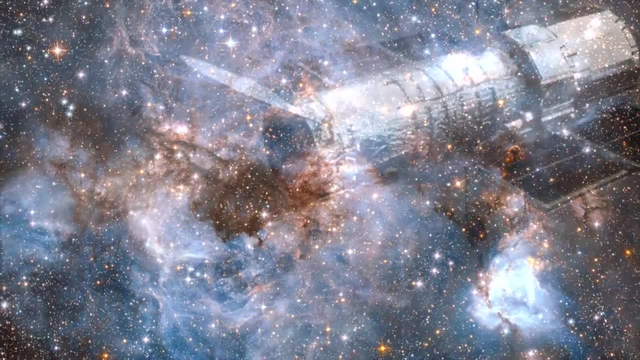 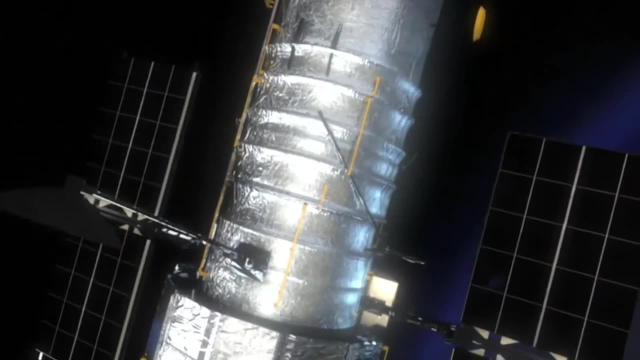 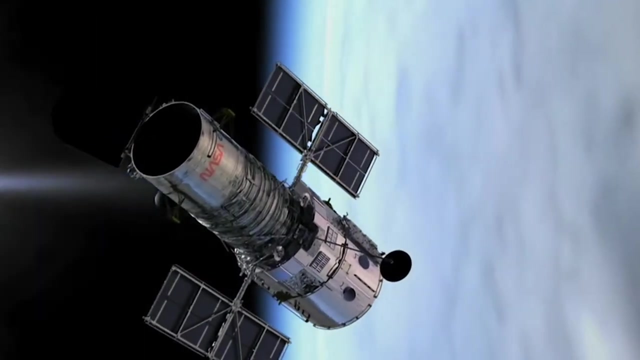 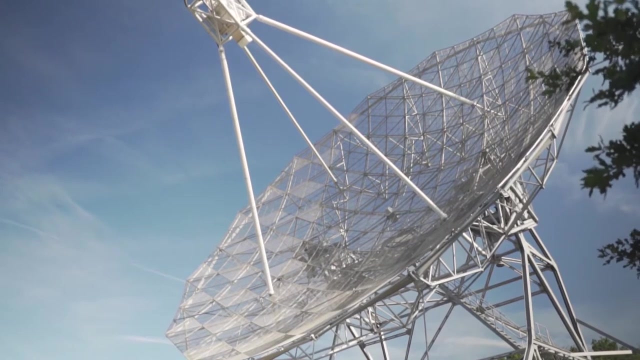 Infrared Astronomy. Infrared astronomy is used to study objects embedded in molecular clouds and the cores of galaxies. Observations from the Wide-Field Infrared Survey Explorer have been particularly effective at unveiling numerous galactic protostars and their host star clusters. With the exception of infrared wavelengths close to visible light, such radiation is heavily absorbed by the atmosphere or masked, as the atmosphere itself produces significant infrared emission. 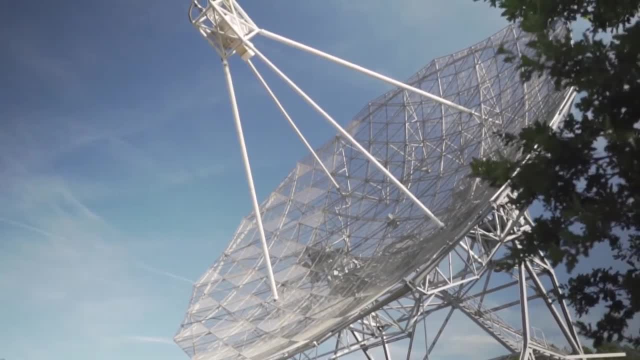 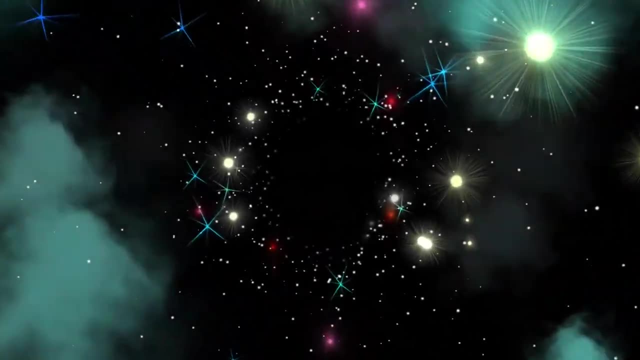 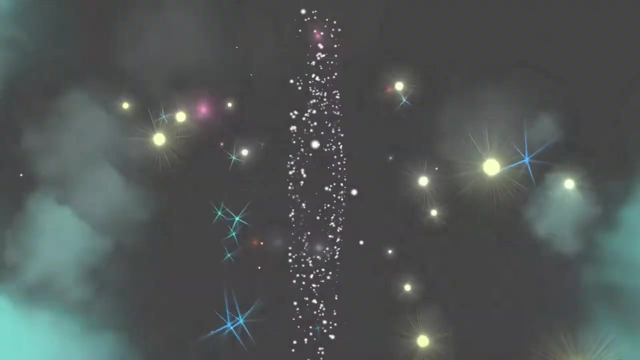 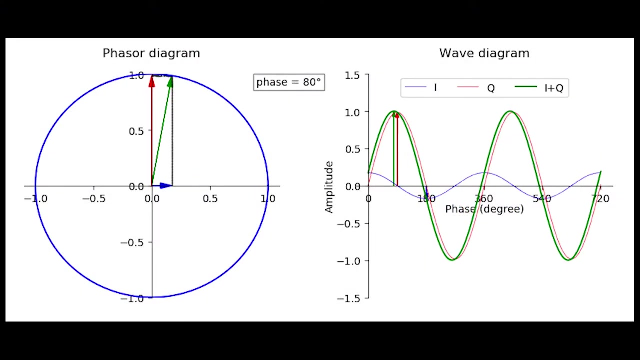 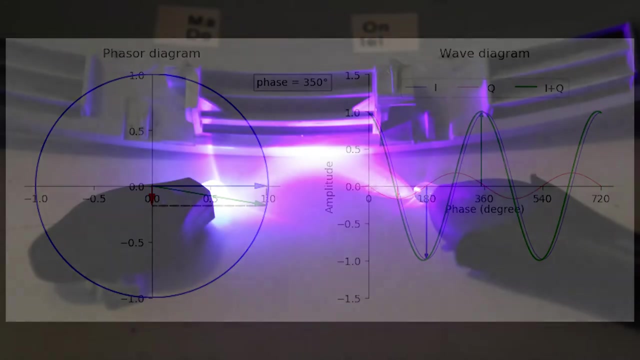 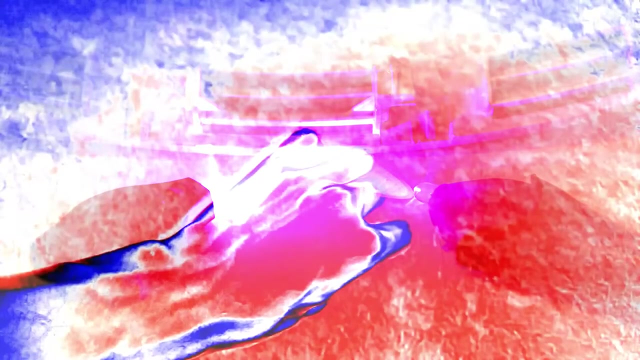 Consequently, infrared observatories have been used to study objects that are too cold to radiate visible light. shot of infrared wavelengths onsecutable Under the Sun: Satellite Array ощ Here. healing мин Flora, Batman, ParId y Se Mei. eren century and most of the 20th century images were made using photographic equipment. 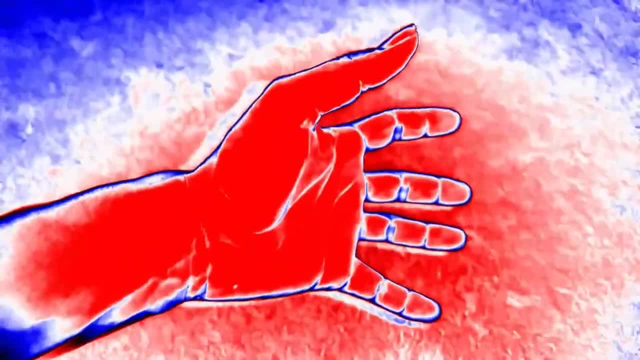 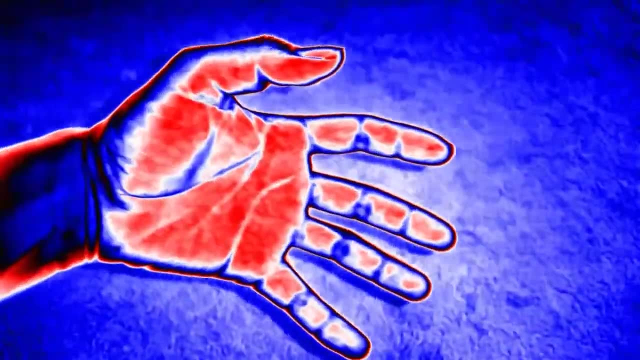 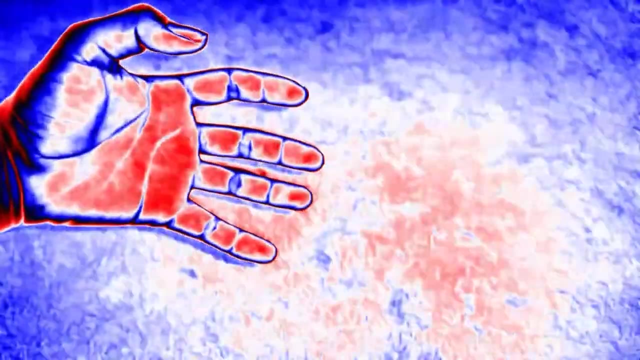 Modern images are made using digital detectors, particularly using charge-coupled devices, and recorded on modern media. Although visible light itself extends from approximately 4000 A to 7000 A, 400 nanometers to 700 nanometers, that same equipment can be used to observe some near-ultraviolet and 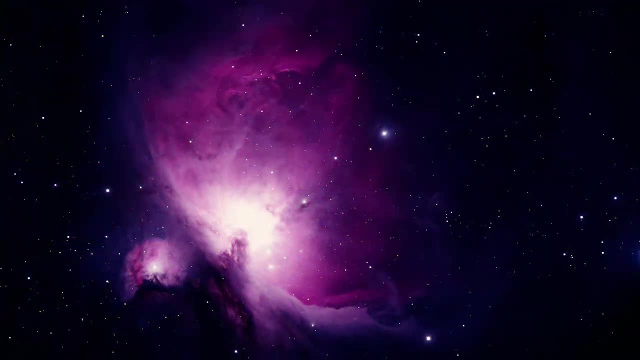 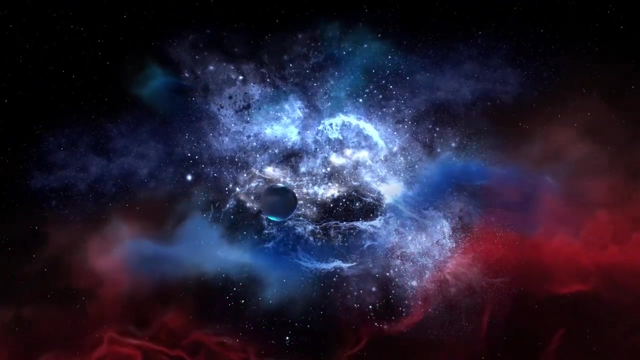 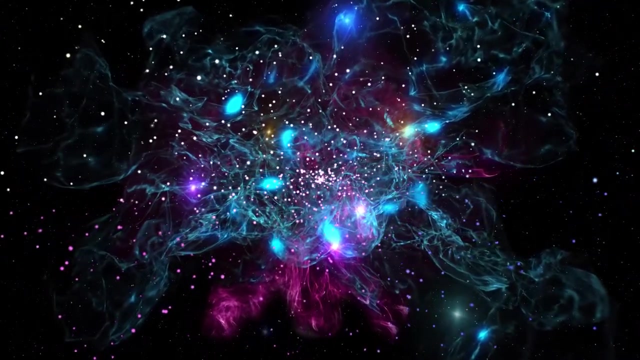 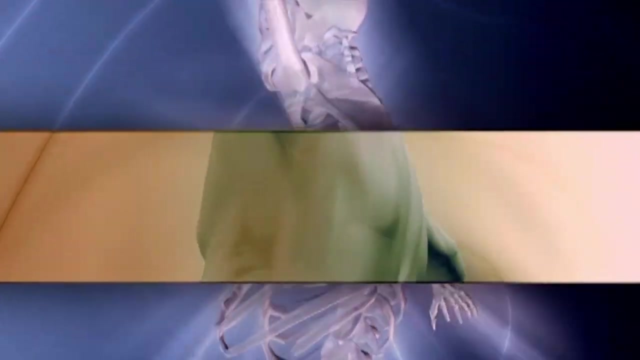 near-infrared radii. Ultraviolet Astronomy. Ultraviolet astronomy employs ultraviolet wavelengths between approximately 100 and 3200 A. Light at those wavelengths is absorbed by the Earth's atmosphere, requiring observations at these wavelengths to be performed from the upper atmosphere or from space. 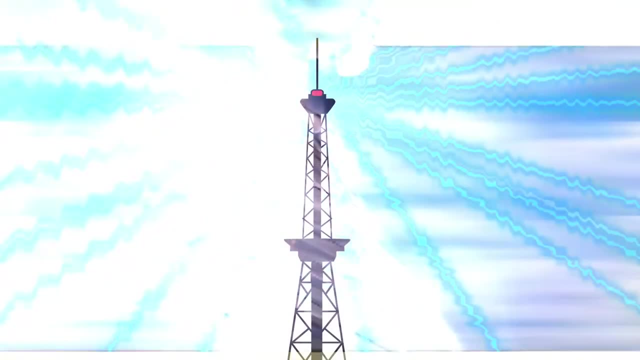 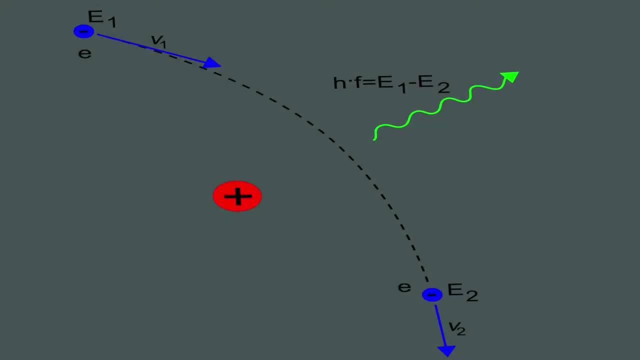 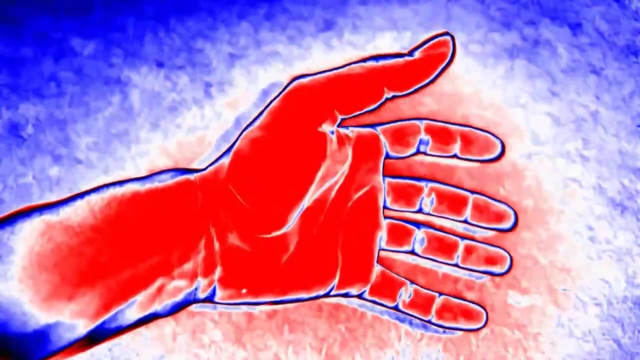 Ultraviolet astronomy is best suited to the study of thermal radiation and spectral emission lines from hot blue stars that are very bright in this wave band. This includes the blue stars in other galaxies, which have been the targets of several ultraviolet surveys. Other objects commonly observed in ultraviolet light include planetary nebulae supernova. 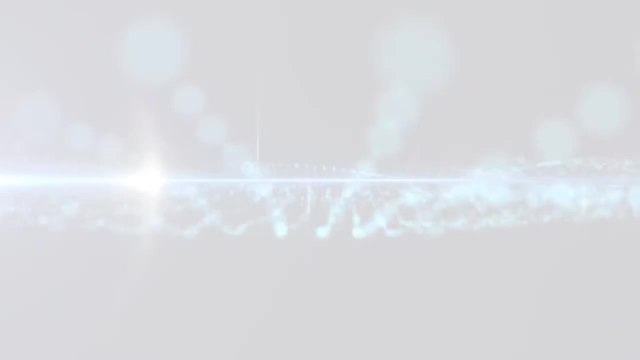 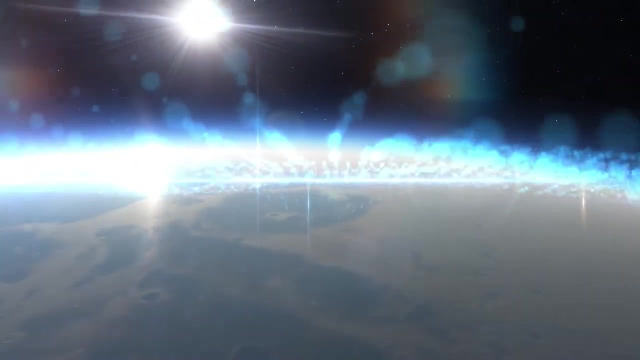 remnants and active galactic nuclei. However, as ultraviolet light is easily absorbed by interstellar dust, an adjustment of ultraviolet measurements is necessary. The light is also used to measure the temperature of the atmosphere. How does X-ray astronomy work? The X-ray astronomy uses X-ray wavelengths. 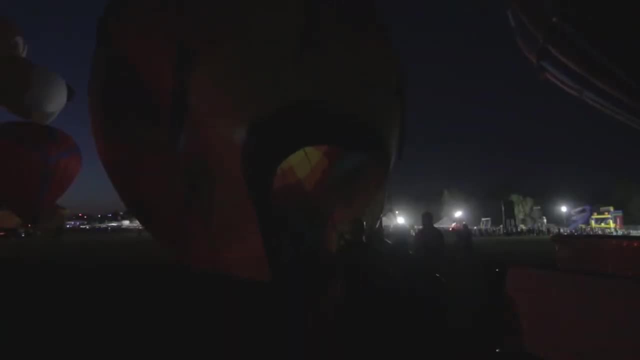 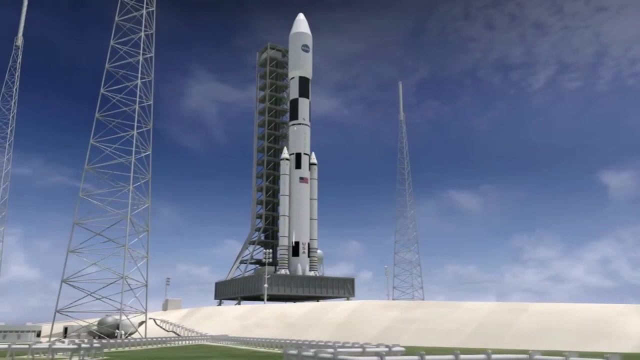 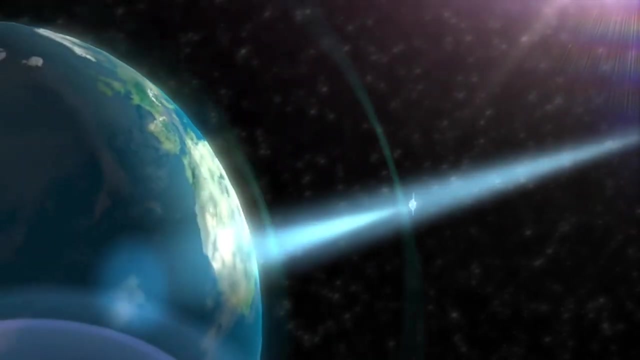 Typically, X-ray radiation is produced by synchrotron emission, the result of electrons orbiting magnetic field lines: thermal emission from thin gases above 107 Kelvins and thermal emission from thick gases above 107 Kelvin. Since X-rays are absorbed by the Earth's atmosphere, all X-ray observations must be performed from. 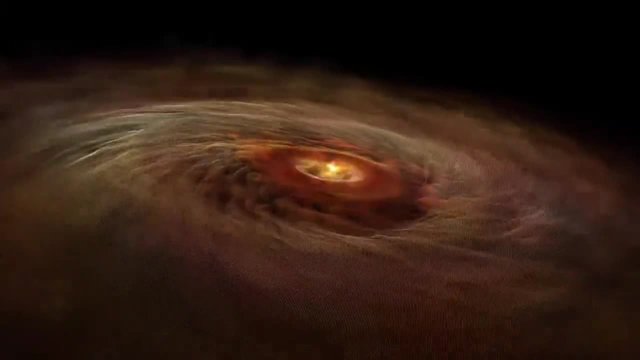 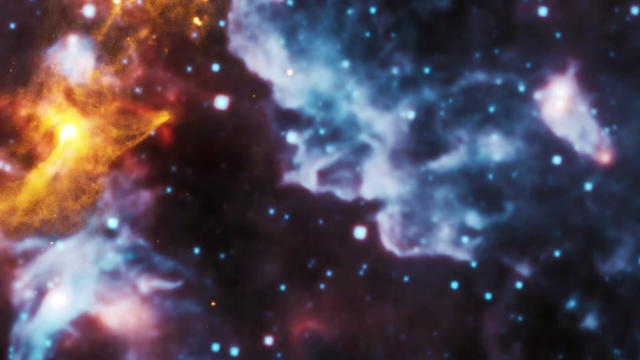 107, Once the X-ray physicians are able to observe them in full depth. the X-ray neurons cannot be opened with a single beam, be performed from high-altitude balloons, rockets or X-ray astronomy satellites. Notable X-ray sources include X-ray binaries, pulsars, supernova, remnants, elliptical galaxies. 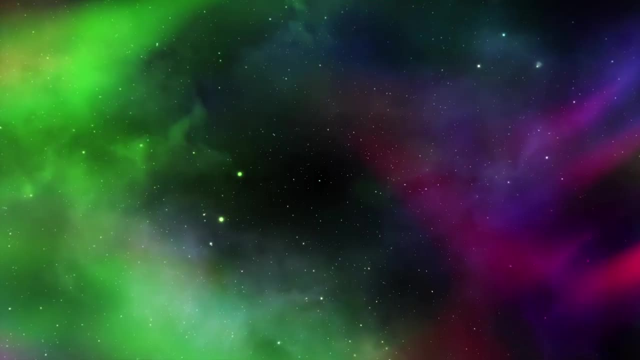 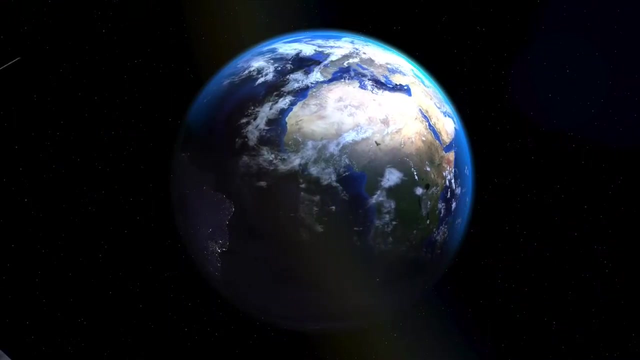 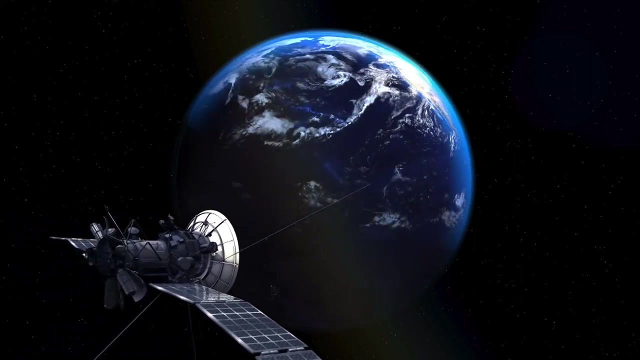 clusters of galaxies and active galactic nuclei. Gamma-ray astronomy. Gamma-ray astronomy observes astronomical objects at the shortest wavelengths of the electromagnetic spectrum. Gamma-rays may be observed directly by satellites such as the Compton Gamma-ray Observatory, or by specialized telescopes called atmospheric Cherenkov. 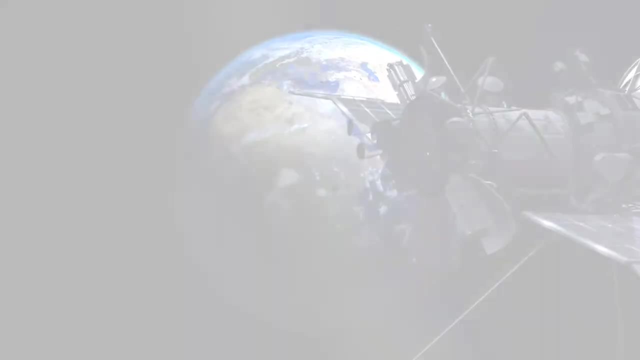 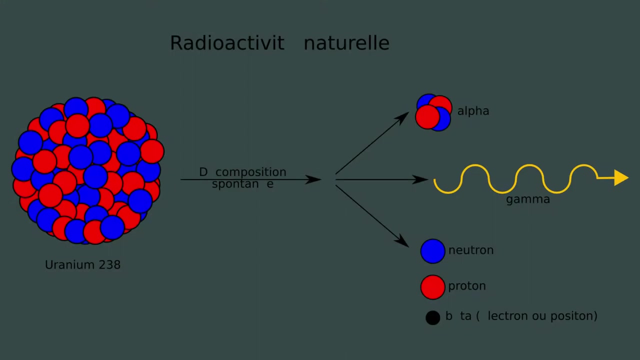 telescopes- The Cherenkov telescopes, do not detect the gamma-rays directly, but instead detect the flashes of visible light produced when gamma-rays are absorbed by the Earth's atmosphere. Most gamma-ray emitting sources are actually gamma-ray bursts objects which only produce 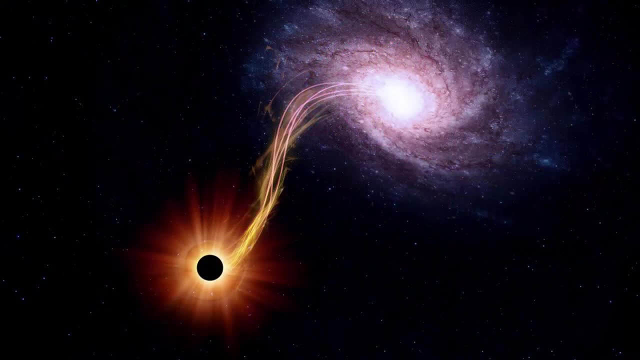 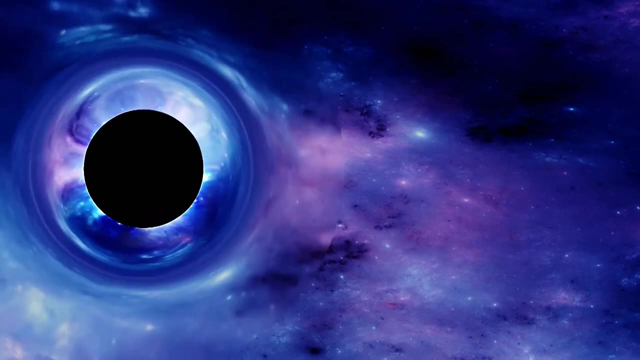 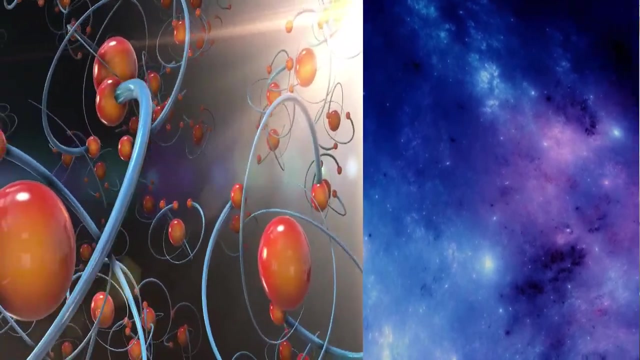 gamma radiation for a few milliseconds to thousands of seconds before fading away. Only 10% of gamma-ray sources are non-transient. These steady gamma-ray emitters include pulsars, neutron stars and black hole candidates such as active galactic nu fields not based on the electromagnetic spectrum. In addition to 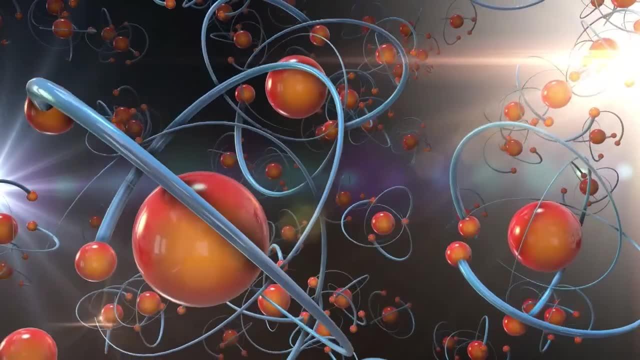 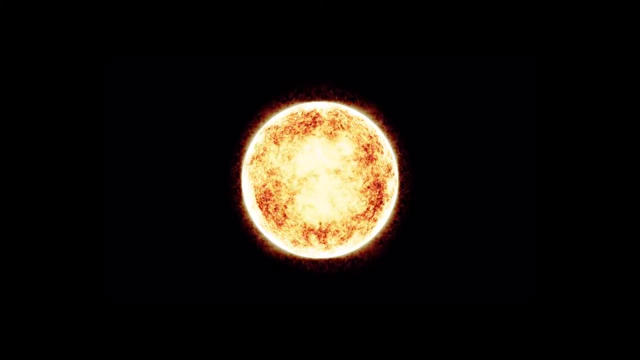 electromagnetic radiation. a few other events originating from great distances may be observed from the Earth. In neutrino astronomy, astronomers use heavily shielded underground facilities such as SAGE, GALAX and Kamioka 2-3 for the detection of electromagnetic radiation. 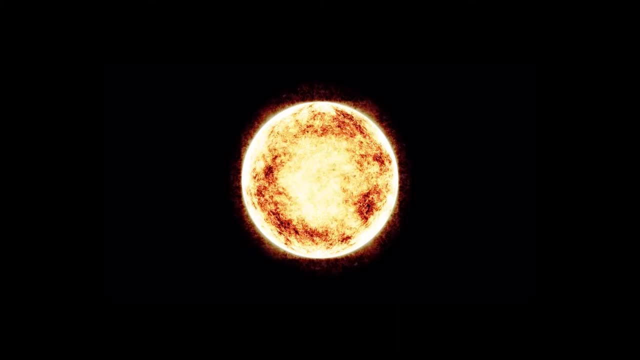 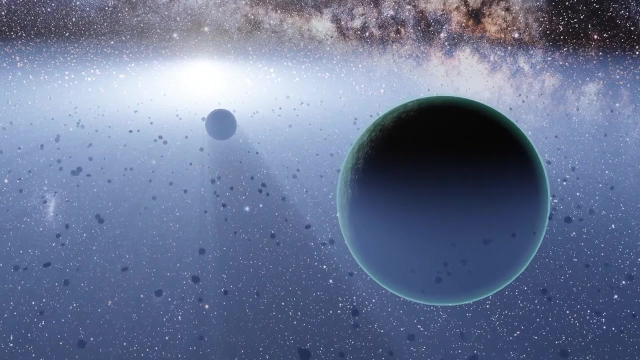 The vast majority of the neutrinos streaming through the Earth originate from the Sun, but 24 neutrinos were also detected from Supernova 1987A- Cosmic rays, which consist of very high energy particles that can decay or be absorbed when they enter the Earth's atmosphere, resulting in a cascade of secondary particles which can be detected by current observatories. 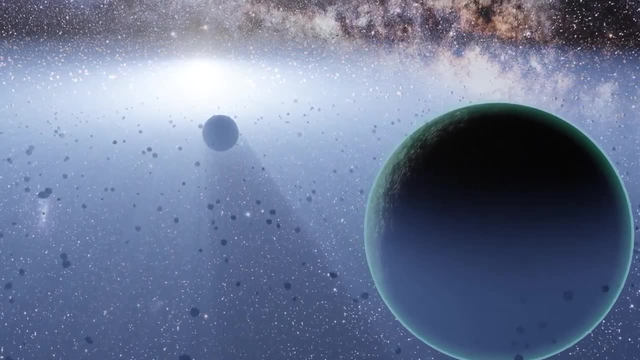 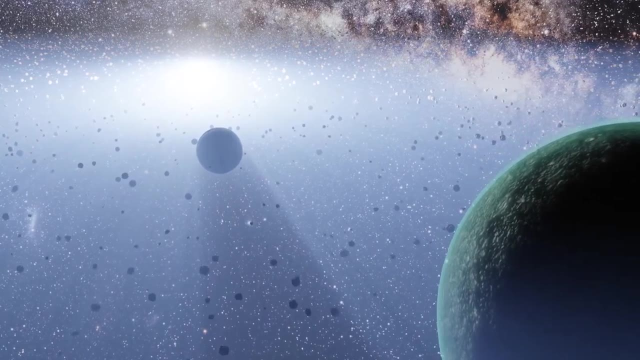 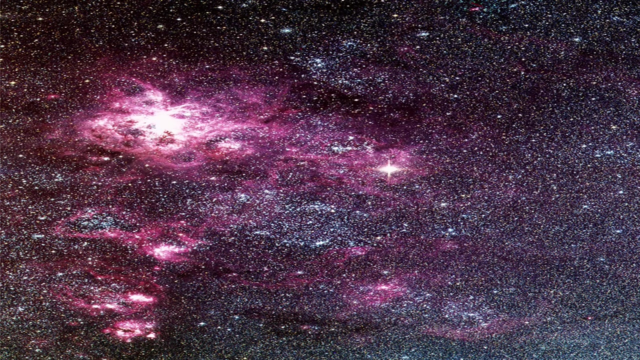 Some future neutrino detectors may also be seen. The gravitational wave is sensitive to the particles produced when cosmic rays hit the Earth's atmosphere. Gravitational wave astronomy is an emerging field of astronomy that employs gravitational wave detectors to collect observational data about distant massive objects. 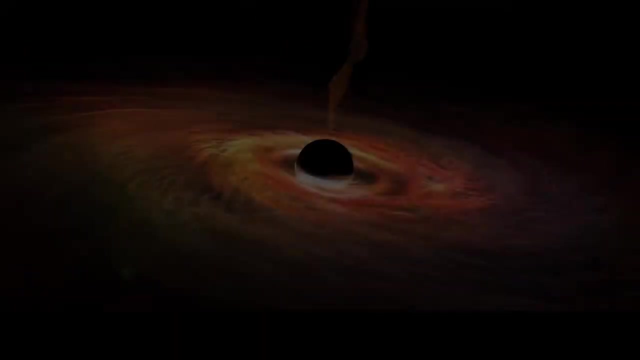 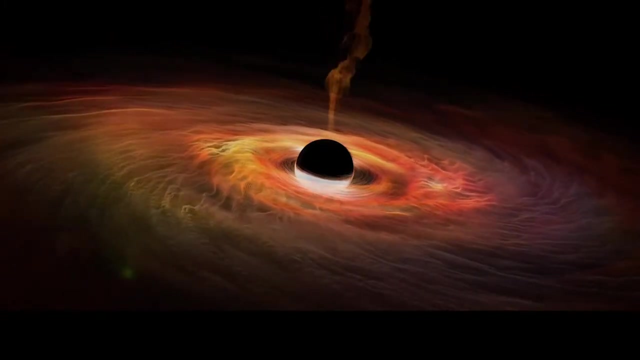 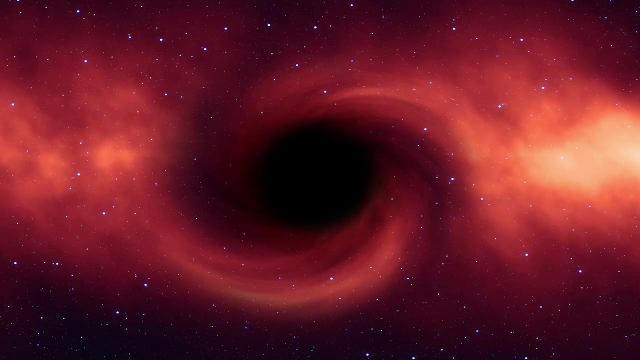 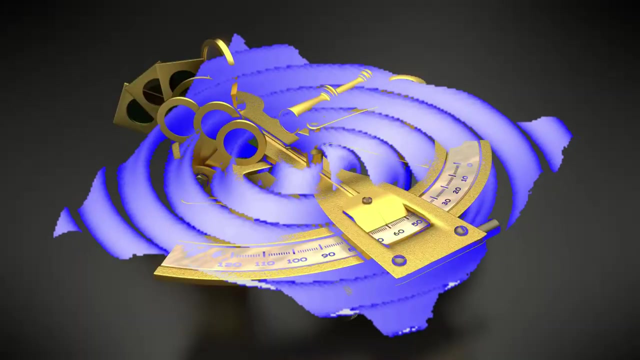 A few observatories have been constructed, such as the Laser Interferometer Gravitational Observatory LIGO. LIGO made its first detection on September 14, 2015,, observing gravitational waves from a binary black hole. A second gravitational wave was detected on December 26, 2015 and additional observations should continue, but gravitational waves require extremely sensitive instruments. 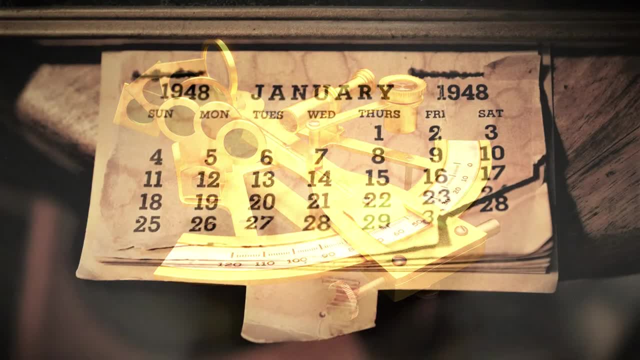 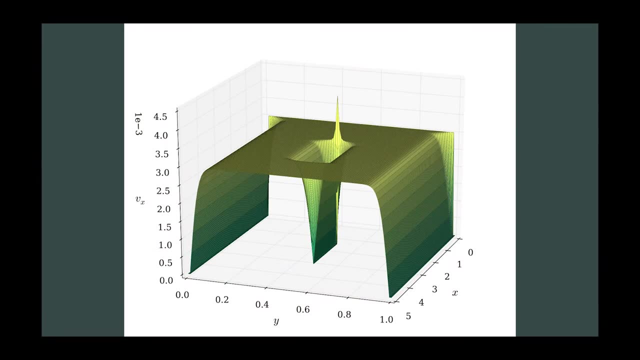 The combination of observations made using electromagnetic radiation, neutrinos or gravitational waves and other complementary information is known as multi-messenger astronomy, ASTROMETRY AND CELESTIAL MECHANICS. ASTROMETRY AND CELESTIAL MECHANICS.